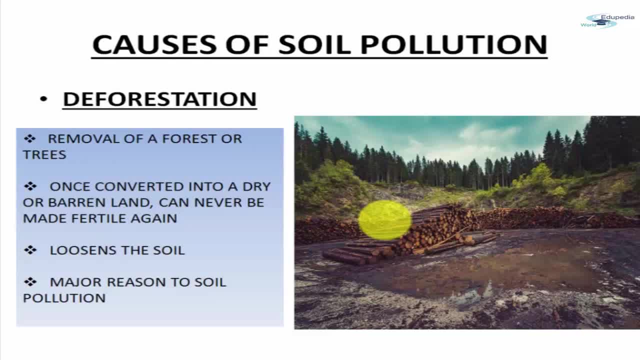 is called as deforestation right. so what happens in deforestation? once they cut down all the trees, the soil erosion takes place. that is because there are no more trees to hold the soil tightly to the ground, so when, when it rains, the soil is just washed away. 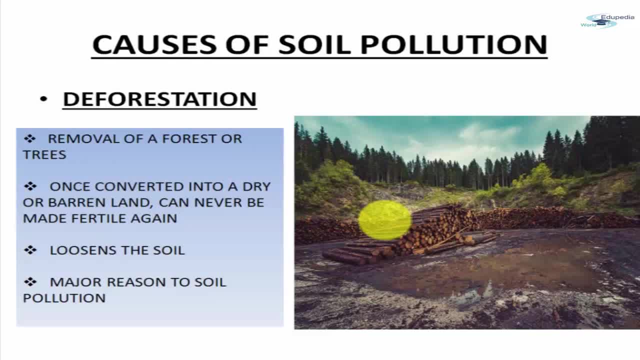 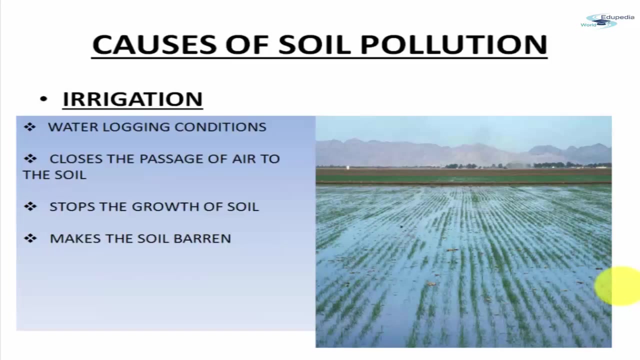 from this area, and this is known as soil erosion. the soil becomes loose right. so this deforestation, the soil erosion, is the main cause of soil pollution, because this washes away all the soil right. so next is irrigation. what is irrigation? irrigation is supplying the water to the crops, or 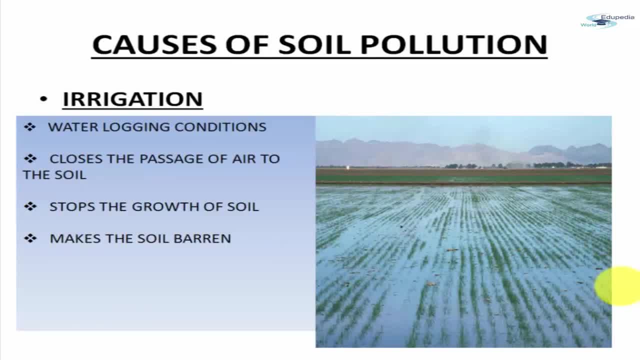 to the fields. but what happens when irrigation- some wrong practices are used for irrigation, similar things happen. this is what you see. this other water logging condition. what happens when we supply water in very, very large quantity than is actually required for the crop, water logging and because of this water, the passage of air toward to the crop or to the field, it stops because of 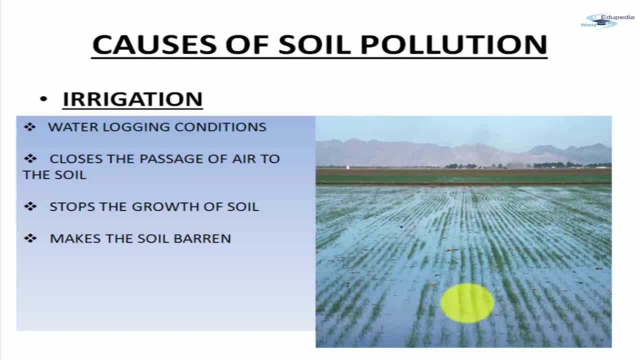 water, air cannot be passed, it cannot be supplied to the crop and because of this, the growth of the crop stops. quality of the crop will be very, very bad, and this over a long period of time. this makes the area barren. it's fertility. so the farmers should know what are the right practices of irrigation. now let's 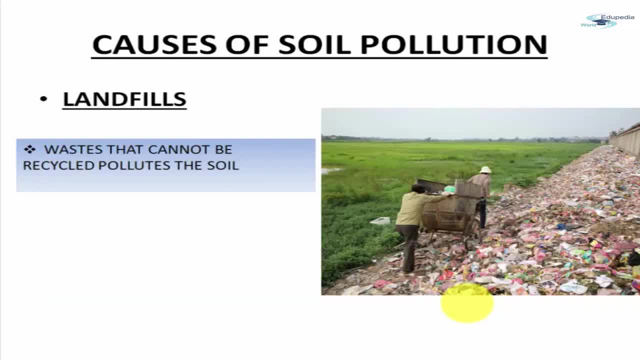 move ahead. landfills. landfills are another way to cause soil pollution. there is a lot of waste. this waste comes out of mainly the houses, the household waste. this creates the. this makes the landfill so these waste also pollute the soil: the agricultural waste, that is, the use of toxic. 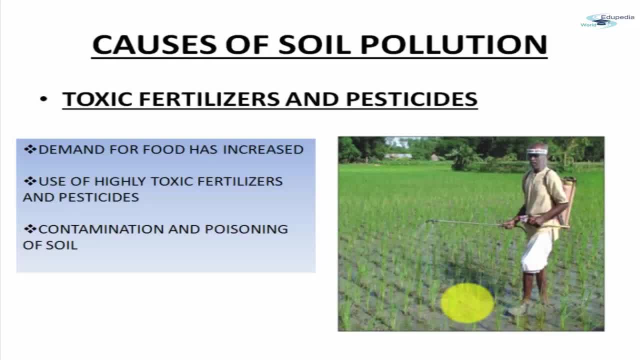 fertilizers and pesticide, they also become a main cause of soil pollution. why, these days, the farmers are using these toxic fertilizers and pesticide? that is because, with the increase in the population, the demand for the food has increased over a period now, because of the increase in the demand, 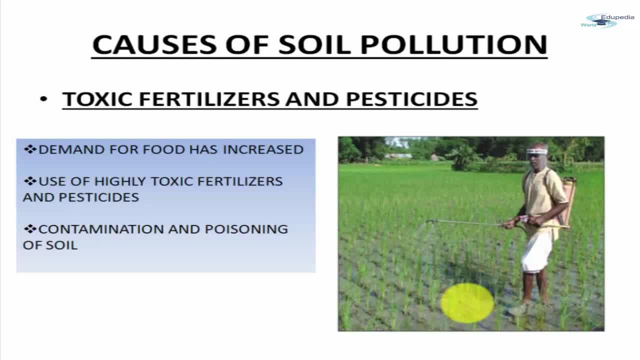 the crop supplies to the landfills are also polluted, so the landfills are also polluted. so the landfills are still the same. the agricultural land will remain the same, but the demand for the food has increased in that short period of time, over that available land, more and more quantity. 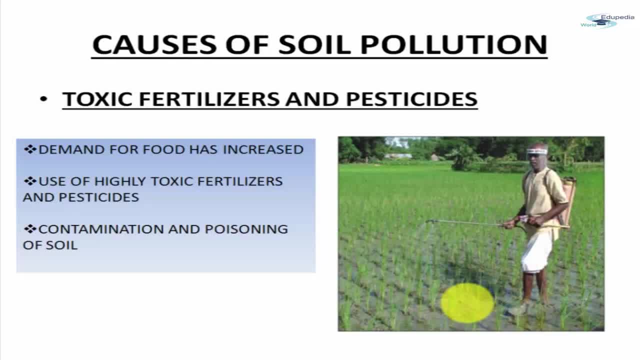 of food is required to be produced, and that is why these days the farmers are going in for these toxic fertilizers and pesticide so that the crop can be produced at a much faster rate. but they do not understand that it has very bad and long-term side effects. so the farmers are going. 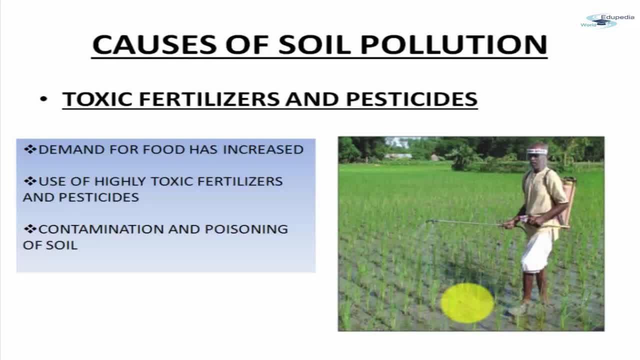 in for these toxic fertilizers and pesticide because what it leads to? it leads to contamination and poisoning of soil. when we consume such a crop, then even we get contaminated over long period of time. this has a very, very harmful effect on the human body. so what is the solution for this? the 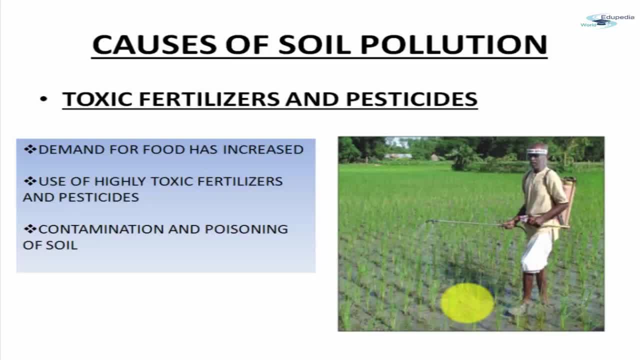 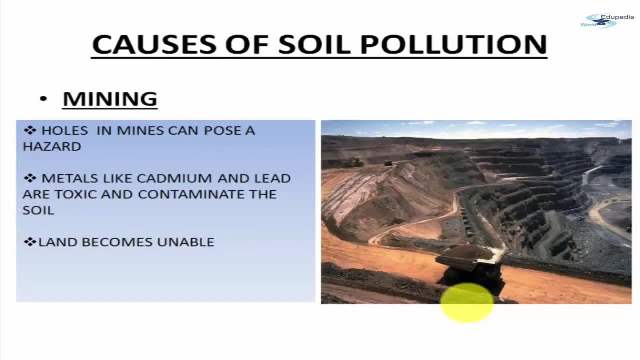 solution is that the farmers should go in for some bio fertilizers, right, okay? mining is another cause for soil pollution and there a lot of harmful gases also. there are a lot of harmful elements which comes out of a mine, which poses a hazard on the human body. also, there are some metals like Cadmium and 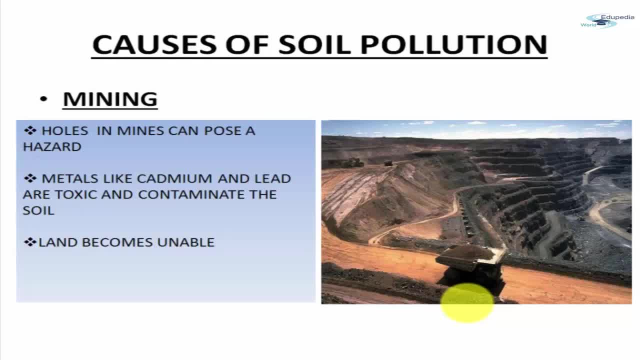 lead, which are very, very toxic, and when they come out of the earth's surface and they contaminate the soil right and the land, as you see here, this is how the land where the mining is done looks like. so the entire land now becomes barren because of such harmful chemicals which are coming out, such 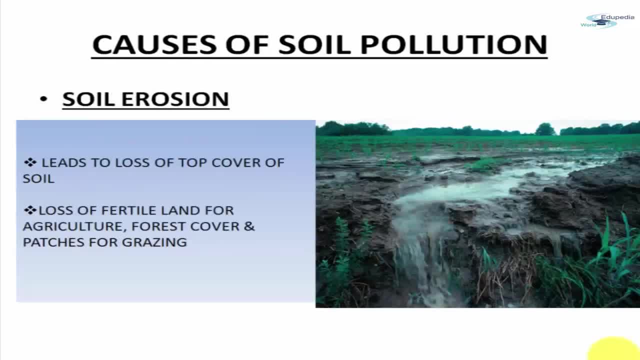 harmful metals which are coming out. the next cause of soil pollution is soil erosion. so this we spoke where when we were discussing about deforestation. now, why does soil erosion occur? how does it happen? when there is rain and there are no trees, the soil is loose, so the entire soil gets, get washed. 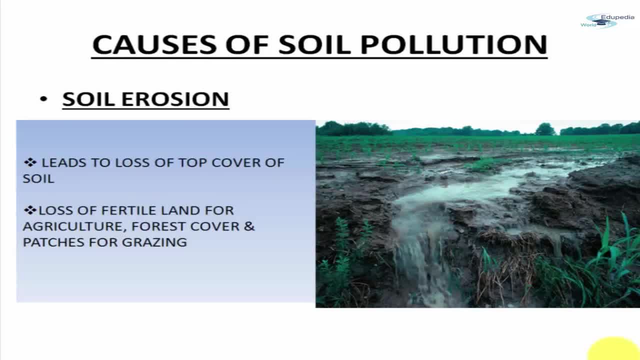 away along with the water, right, and with this soil, a lot of good nutrients, which are required for good quality crop, are also washed along with the water. that is why it affects the quality of crop. that is why- because now there are no nutrients left in the soil to produce good quality crop, the 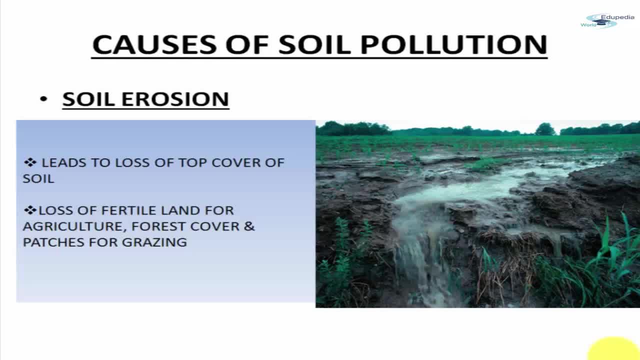 quality of the crop will be down. the quality of the crop will be bad. this is what is called as soil erosion. so soil erosion leads to loss of fertile land for agriculture. it leads to, you know, loss of forest cover and also patches for grazing, that is, grazing for the animals, the kettles, right? so that is what is known. 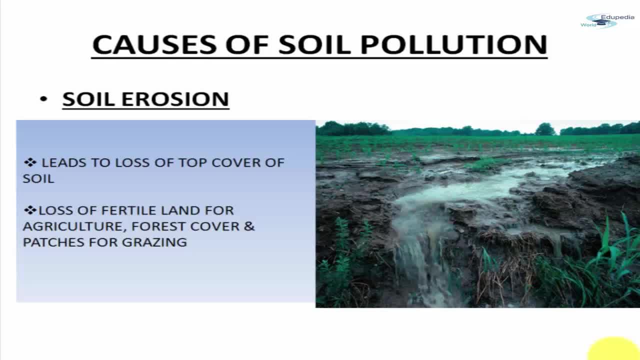 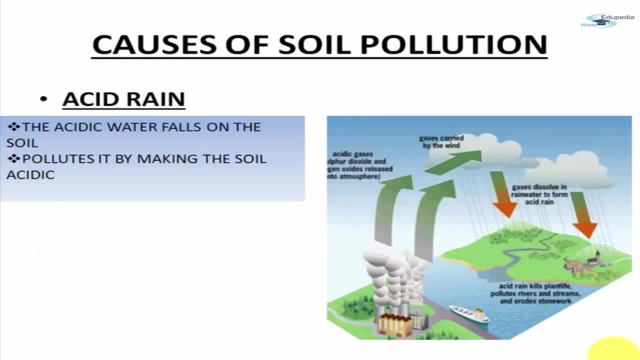 as the soil erosion which is the which is also one of the cause for soil pollution. okay, next is acid drain. acid rain also pollutes soil. what is acid rain? see acid rain. it is also a product of the waste that comes out of our land. and then you look at the collector bringing that use of acid rain. 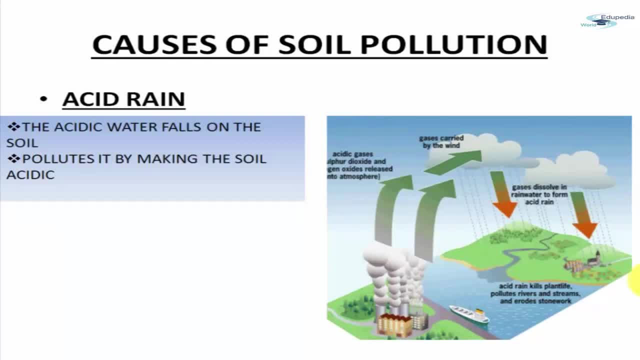 that comes out of the industries, right? so these are, let's say, these are the industries and the gases. the harmful gases that comes out of the industries are sulfur dioxide. these are nitrogen oxides. so the basically sulfur dioxide and nitrogen oxides are the two gases which are very, very harmful, and these 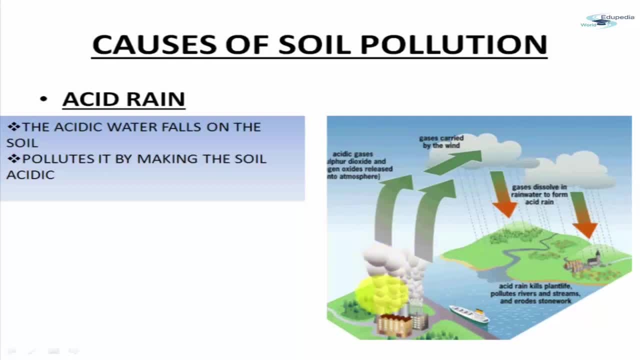 are what comes out of the industries. so when these acidic gases are released in the atmosphere, the gases are. then these gases are carried by the wind and then they become clouds here. so now these clouds contain these harmful gases. ultimately, when the precipitation, when it rains, then these harmful gases are. 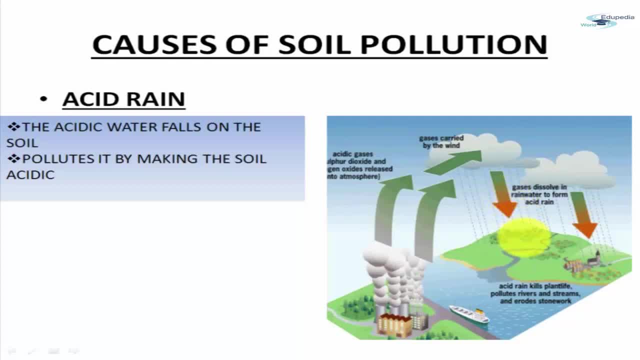 dissolved in drain water and when it falls on the surface of the earth, then this is what is called as acid rain. acid rain can kill the plants, they can pollute the river, the rivers, the streams, right, so this is how the acid rain is very, very harmful. so acid rain is also the main cause for 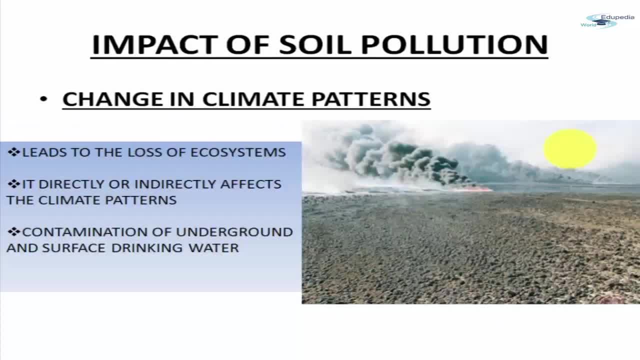 soil pollution. so now we are going to talk about impacts of soil pollution. till now we have talked about what does soil pollution and what are what causes the soil pollution. now, because of these causes, what? what happens? what are the impacts of soil pollution? so the first impact is the lignite european soil paint. the last, biggest, cinco, ganska: 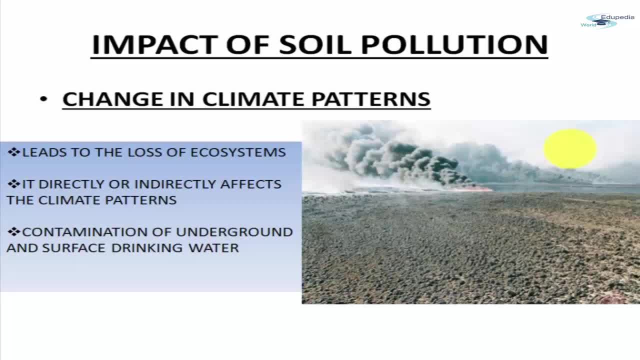 is change in climatic patterns. Now we have been seeing that because of acid rain, the lights that lives on earth's surface and even the marine life which lives in the water. everything gets affected. Everything has a harmful effect on their body if they are exposed to such kind of acid rain and 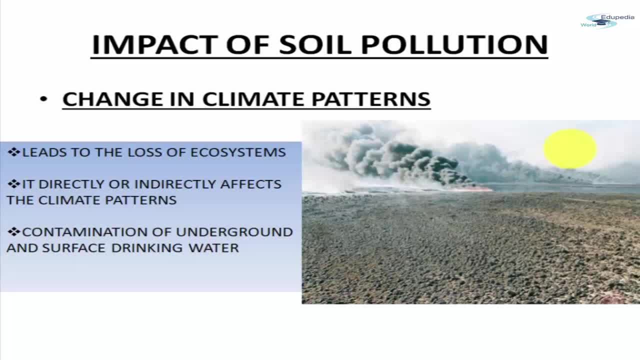 such kind of contamination for a long period of time. So neither the land, nor water, nor the air, nothing is pure. Everything is contaminated. So this kind of pollution is ultimately changing our climate. The climatic patterns are changing. Why? Because the entire ecosystem is changing. 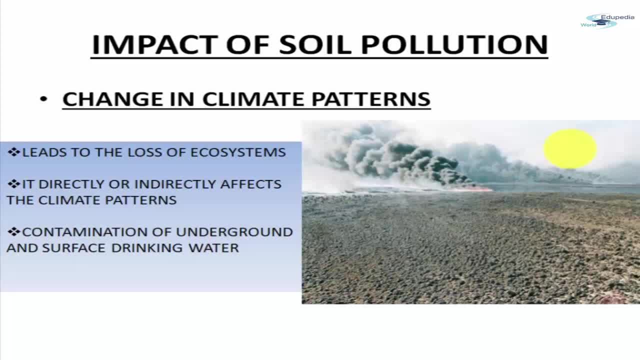 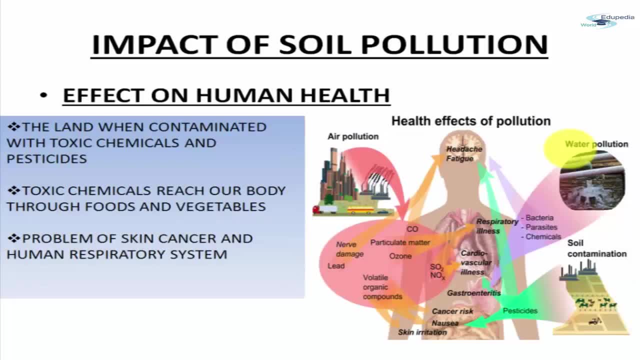 The entire ecosystem is contaminated. So that is what I mean when I say change in climatic condition. Next and major impact is impact on the human health. What is the impact on the human health when the land gets contaminated? there are a lot of toxic chemicals and pesticides which enter 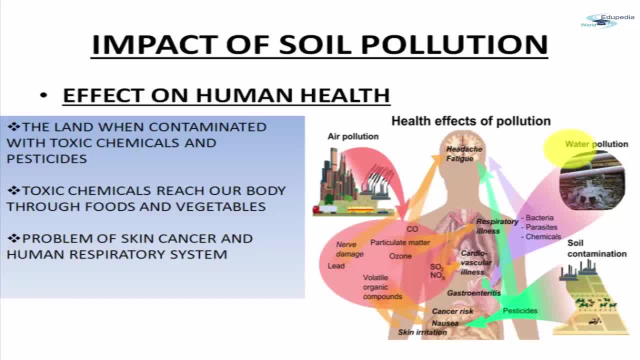 which comes on the earth, which enters the soil. so when we human beings or the animals, when they eat such crop or such agricultural product, then even those chemical, harmful chemicals get into their body and over a period of time they will have some harmful effects they will. they may have a skin problem, they may have respiratory problem if we keep consuming. 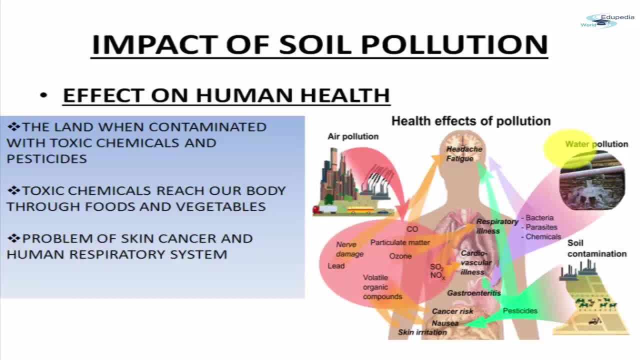 such harmful crop, it starts from a very, very minor problems and then it leads to major problems. we have air pollution continuously. we have water pollution. we also have soil contamination right now. because of air pollution generally, we have problems in respiration and water pollution will have a lot of disease, like you know: typhoid. 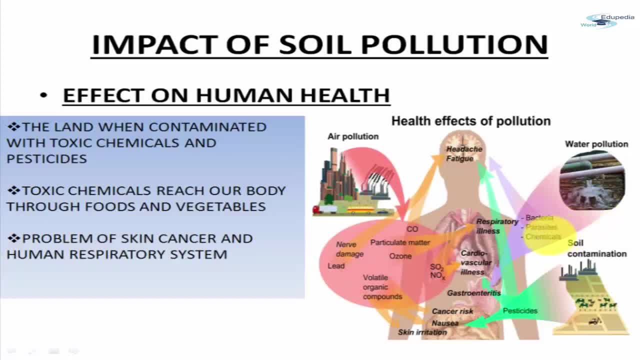 and a lot of bacteria and parasites and other chemicals that are entering in our body. so then again, because of soil pollution, we end up consuming harmful pesticides in our body. so we have problems like skin irritation, nausea, cancer risk, gastrointestinal and cardiovascular illness, respiratory problems. so all these three, that is all the pollution, the soil pollution, the. 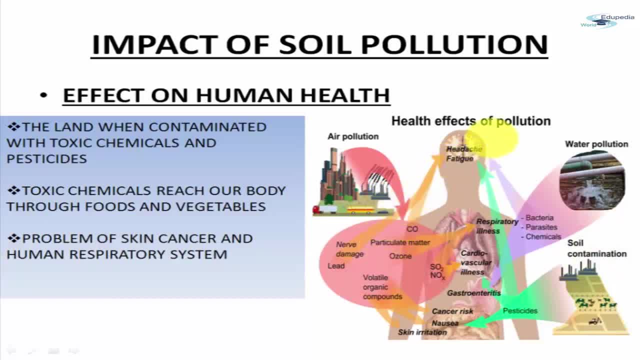 water pollution and the air pollution all together causes the headache fatigue, right. so if we are exposed to such a contamination for a long period of time, then it has a very, very harmful effect on the human health. so next is impact on the environment. with deforestation, the 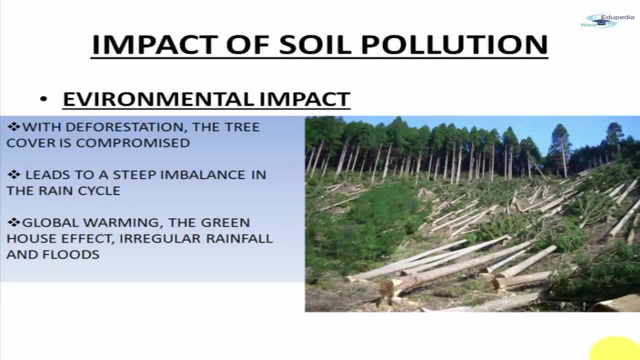 trees are cut down and the tree cover is also compromised. so when there are no trees, there are two things which tend to happen. first is that soil erosion will take place, that is, the top layer of the soil will be washed away, and second thing is that it imbalances the rain cycle because of because of no trees. 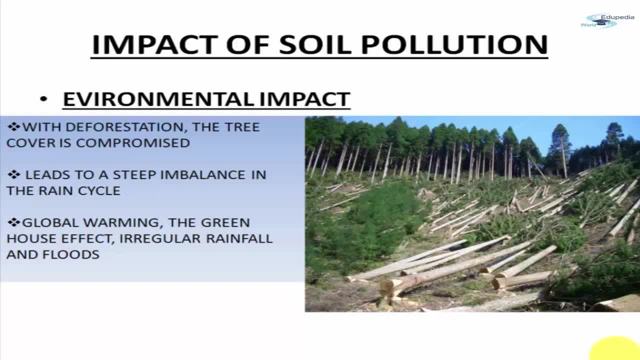 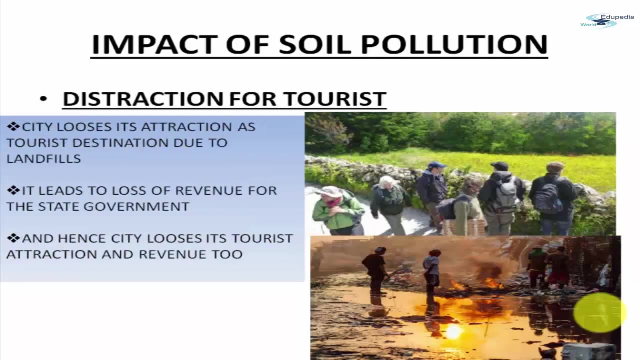 there won't be any more rains right and with this imbalance there are other imbalances in the nature which will happen, for example, the global warming, the greenhouse effect, irregular rainfalls and recent floods. so these are few more imbalances with which tend to happen. if deforestation continues, next impact is distraction for tourists, not just. 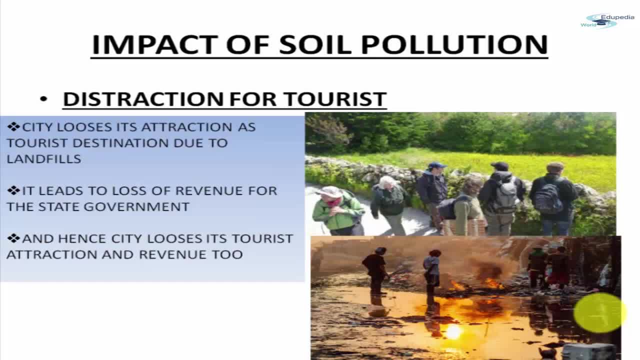 imagine it: there is one city which is neat and it is known for its beautification. on the other hand, there is another city which is full of landfills, and it has. it is polluted because of air pollution, dirty water everywhere, landfills everywhere and dirty environment. so which one do you think that the tourists would like to visit? definitely. 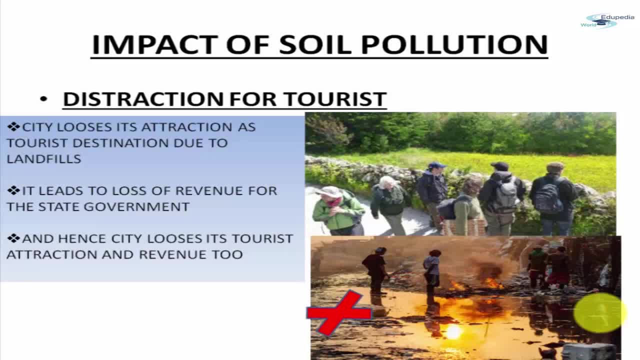 not, which is, which is full of landfills and it has pollution everywhere. tourists generally gets attracted to a city which is neat and clean and it is beautiful. so because of soil pollution, such cities loses its attraction as tourist destination due to the pollution everywhere and as the tourist. 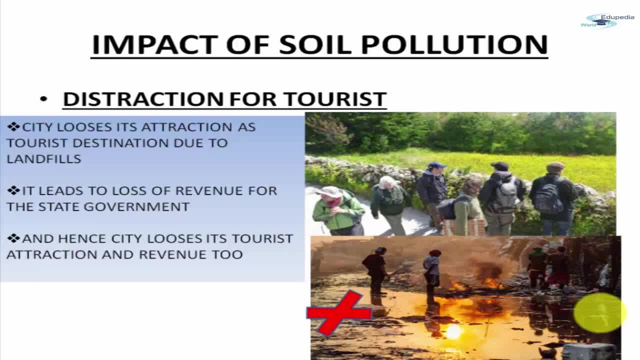 would reduce because of pollution. this leads to loss of revenue for the government also, and hence, on the other hand, even the city loses its attraction and revenue too. so distraction for tourists is also another impact of soil pollution. so now we talked about impact of soil pollution on human health, but 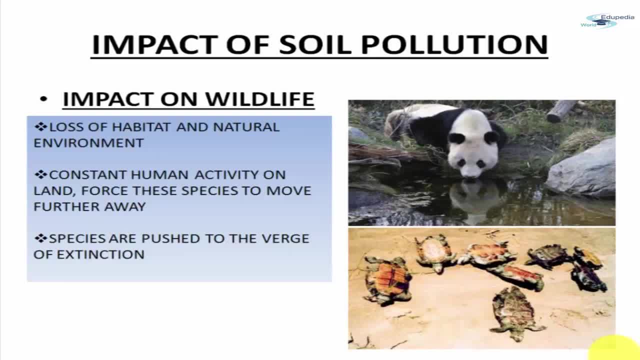 it is not just the human health which is affected because of soil pollution, but even the wildlife is affected. and how are they affected? let's say, if any animal is drinking a water and this water is polluted because of pollution, then the animal will have harmful effects on on his body after a long period. right the 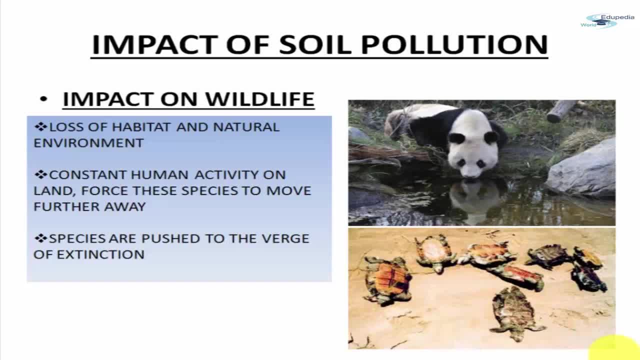 animal might shift to a new location where he could find drinkable water and safe environment to stay. This soil pollution also leads to lot of loss of habitat and natural environment. There are some of the species that are almost coming to an end. They are almost extinct now. 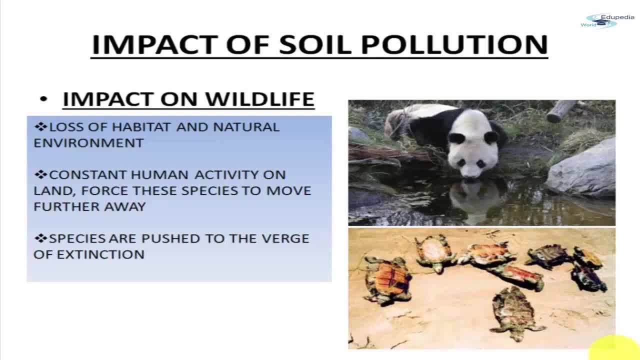 That is the real cause. the actual cause for their extinction is also pollution. Most of the animals and the kettles and the other marine life they die because of lot of contamination in the water or on the land. So the soil pollution may also lead to death of any animal or the wildlife. 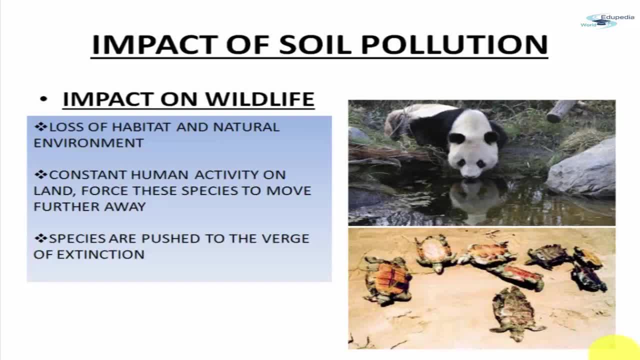 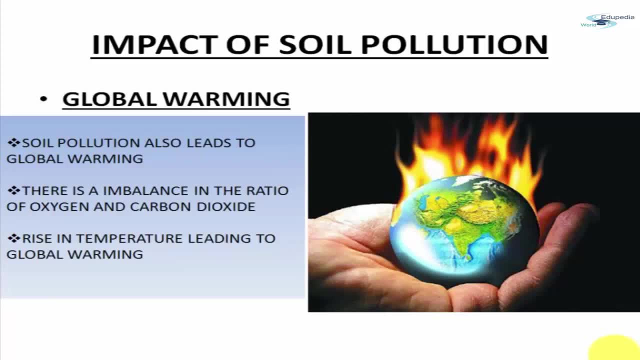 So these are some of the impacts of soil pollution on the wildlife. Now we talked about various imbalances in nature, and one of those imbalances we spoke was global warming. Soil pollution leads to global warming, and what is global warming? Global warming is the increase in the amount of carbon dioxide in the environment. 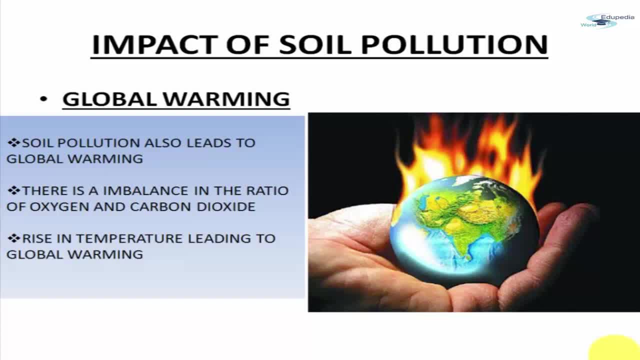 around the surface of the earth, And the main cause for this global warming is pollution. So the ratio of the carbon dioxide and oxygen, the balance between the oxygen and the CO2, is again imbalanced, And this increase in the CO2 gives rise to very, very high temperature. 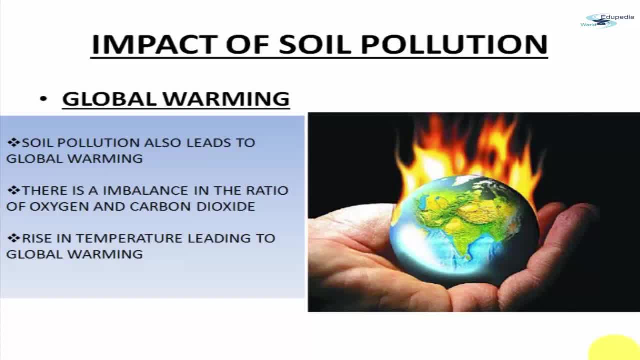 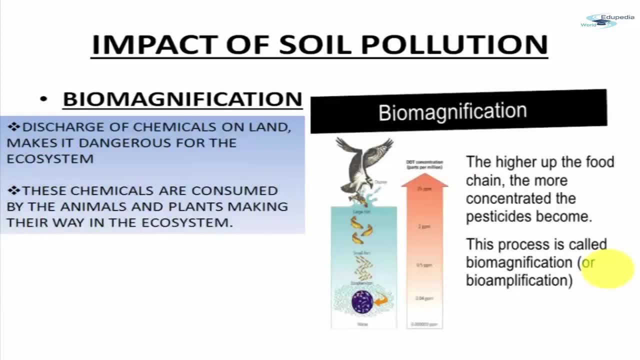 So this is called as global warming. This rise in the temperature actually leads to global warming, which is not a safe environment to stay in. Next is bio magnification. What is bio magnification? It is the transfer of the harmful chemicals from one body to another body. 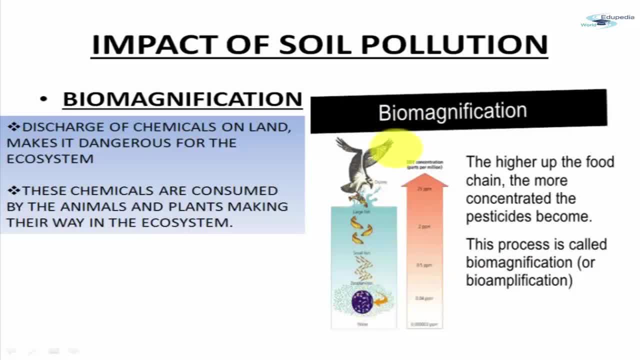 Let's say, as we see here, we have food chain which is shown over here, Smallest organism to the largest organism. The chemicals are transferred because the primary producer is consumed by the zooplankton. The zooplankton are eaten by small fishes. 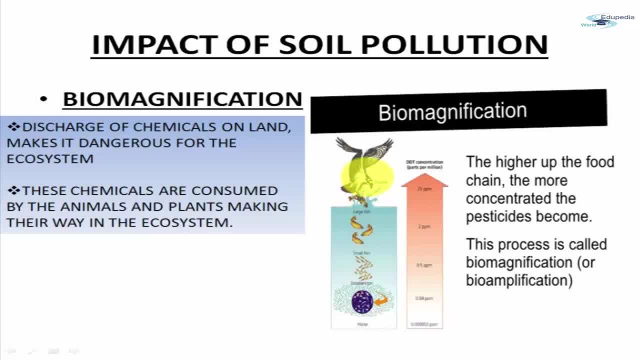 The small fishes are eaten by the large fish and thereafter they are eaten by the eagle or the tertiary consumer. So this way, these harmful chemicals that were initially present in the water, they are consumed and they are transferred to the tertiary level. So this is called as bio magnification. 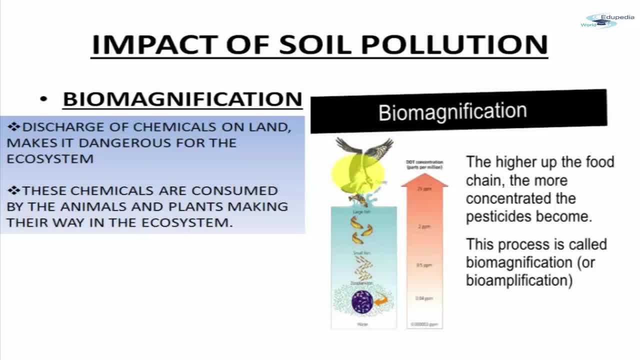 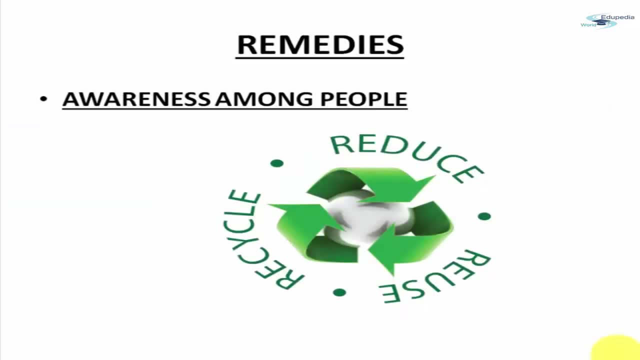 The discharge of chemicals on the land. This makes it dangerous for the ecosystem. So it is basically the transfer of these harmful chemicals from one level in the food chain to the other level. So now let's just discuss the various remedies of soil pollution. 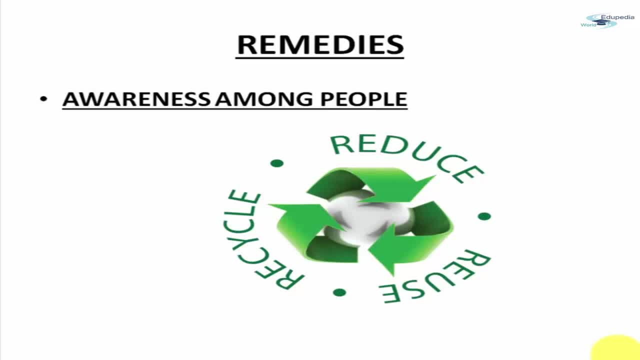 How can we reduce soil pollution? First and foremost is that people have to be aware about the quality of the soil. This is the most important thing. People have to be aware about the quality of the soil, the concept of- you know, reuse, recycle and reduce. This concept we have talked about in the earlier 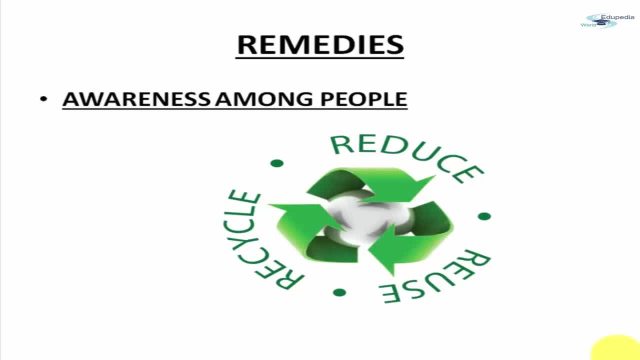 videos also. Only if people are aware about this concept, they will be able to effectively use the products which are eco-friendly and they will be able to avoid such products which are non-biodegradable, like the plastic. And also the awareness should be about: you know what are the. 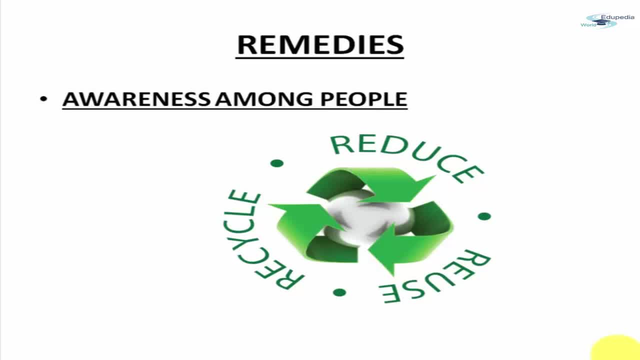 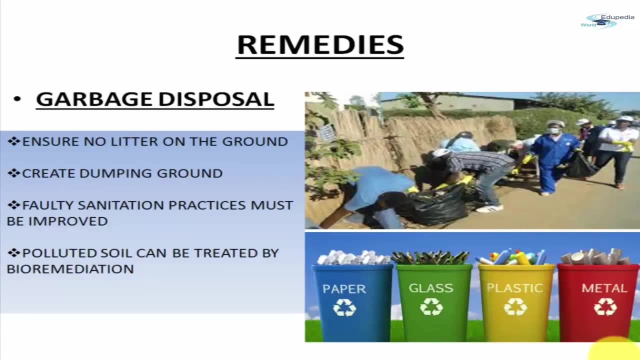 causes of soil pollution? how can it affect our human health and our ecosystem? So only if this awareness spreads among people, they will be more cautious towards the soil pollution. So next solution is garbage disposal. That is, what do we mean by garbage disposal, That is, disposing of. 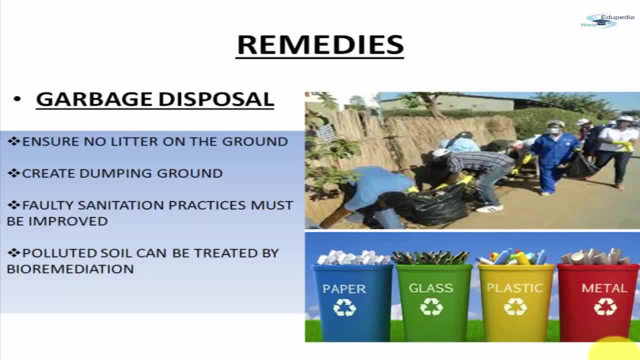 garbage. First of all, the garbage has to be disposed of properly. In case there is any litter which is lying outside our house or nearby area surrounding, then if it is lying in open, then it has to be picked up and disposed of properly in proper garbage bins. Secondly, we have to create dumping grounds, That is: 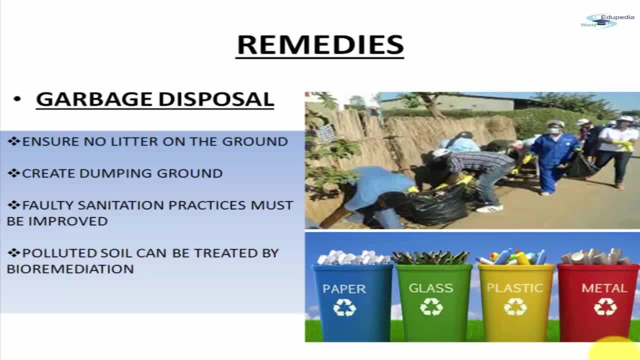 these dumping grounds should have a specific place where the entire garbage is to be dumped. Now also, we see that in most of the localities, they make a dumping ground wherein the garbage from each house is picked up and it is dumped in that area. Right, so this is how proper dumping grounds has to. 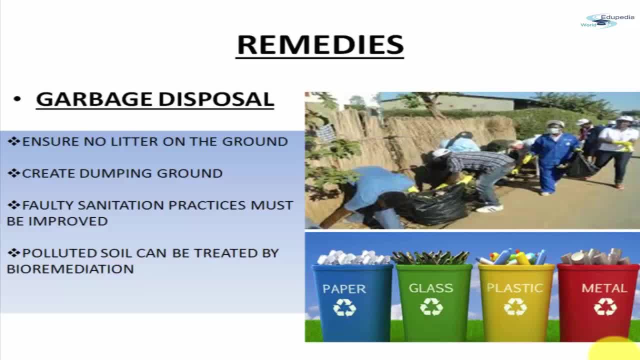 be created for garbage Faulty. sanitation practices must be improved. That is in case in like in earlier days we have seen people are used to go and in open fields for sanitation. So those practices have almost stopped but but still we see that in villages and other rural areas People are still 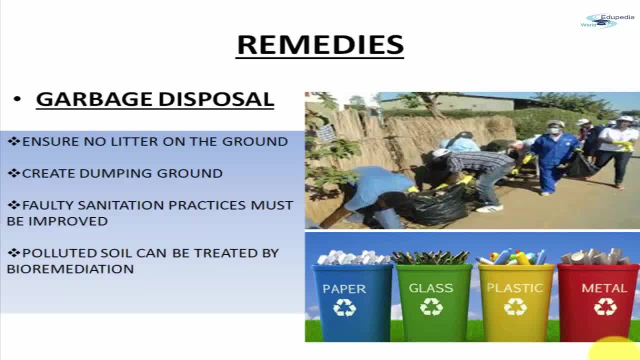 following the same sanitation practices. This has to stop. the toilets have to be constructed. In this picture, as we have seen, people are using proper plastic bag, which are the garbage bags, and then they're picking up the garbagess, putting in these plastic bags, and then these plastic bags will be thrown in proper dumping grounds. So 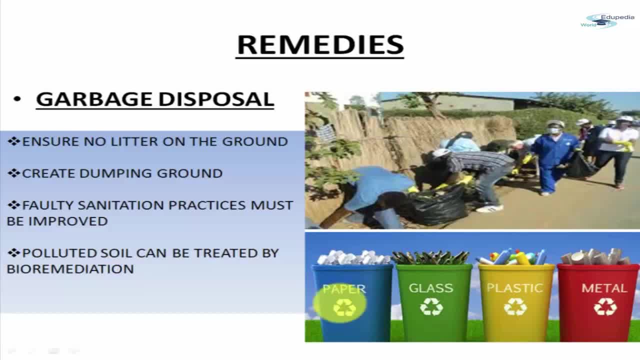 that is how the practice has to set in. Also, we see that different kinds of these bins are used for various garbages, like: if it is a paper, then it has to be thrown in a separate bin. If it is glass, it is plastic, because plastic is again non biodegradable, and then metal. But these are 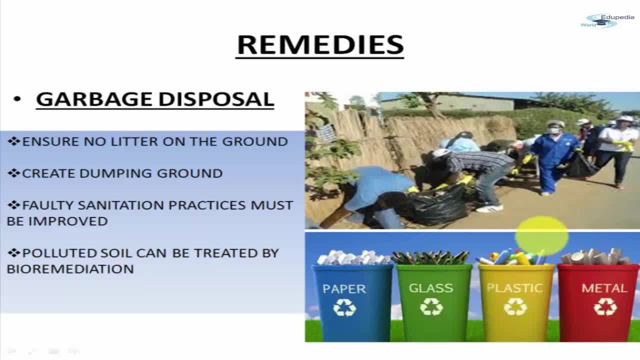 generally done in hospitals and other industries, But at home what we can do is that we can separate the dry and the wet waste. Two bins has to be used. One bin should be for dry waste and the other bin should be for wet waste. The wet waste may be used to produce or create. 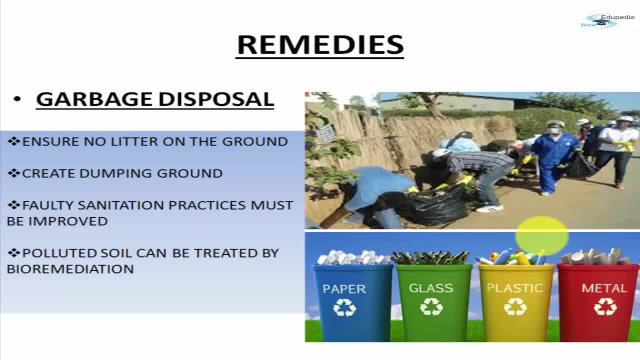 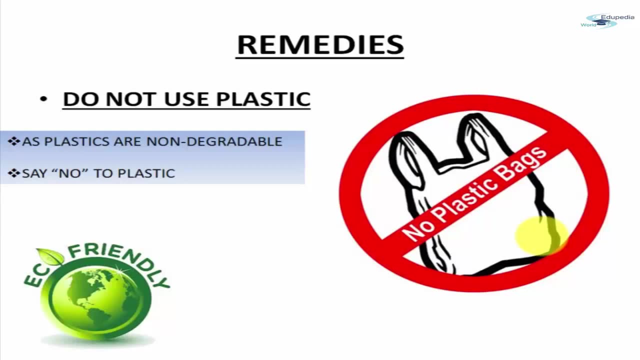 manure which can be used in fields and other agricultural practices. So this way we have to know good practices of garbage disposal. This is very important and we have reiterated this point in our previous videos. also, Do not use plastic, because plastics are non biodegradable- They cannot. 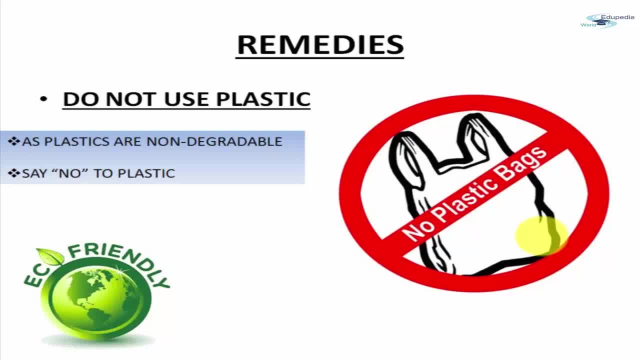 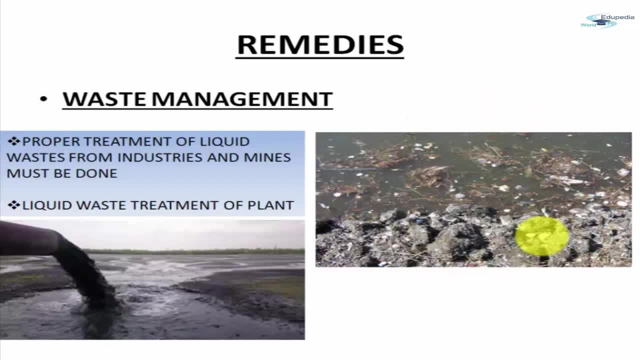 be recycled and also they are not eco friendly. So we have to say no to plastic Again. waste management: it is almost equal to what we discussed about garbage management, But garbage management is mostly out of the question, So we have to know good practices of garbage disposal. This is very 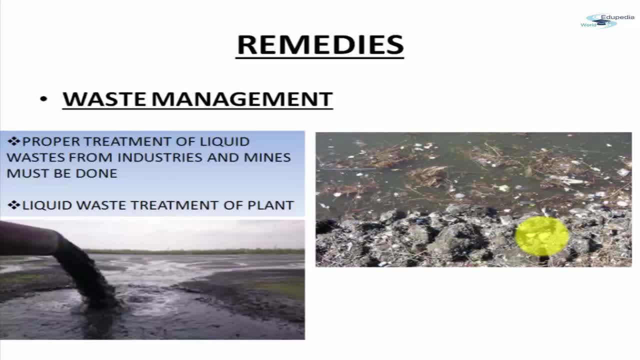 important Waste management is. here we are talking about the waste which comes out of the industry, Proper treatment of the liquid waste which comes out of the industry and mines. this must be done When this water or these kinds of waste, when they are added to the natural water resources, then they 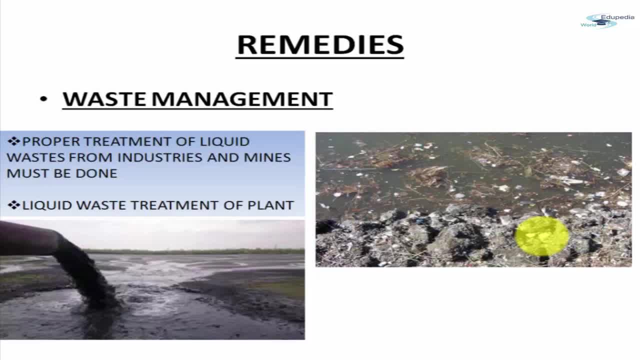 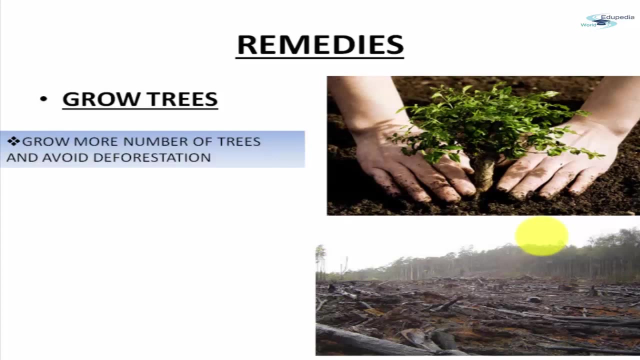 make these water resources dirty. There is a lot of pollution that is created because of these liquid waste. So before the liquid waste from the industry and mines comes out and it mixes with the natural resources, it has to be cleaned properly. Liquid waste treatment of plants has to be done. Very, very important is to grow trees. The more number of trees we grow. 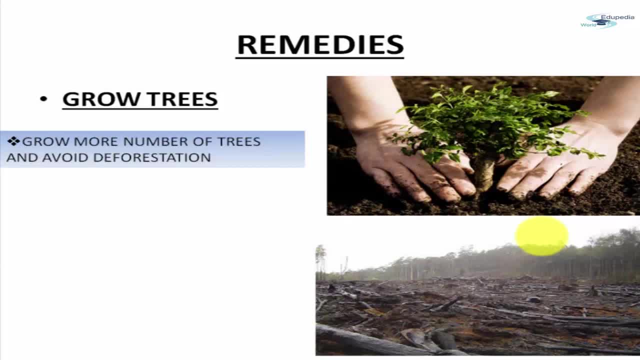 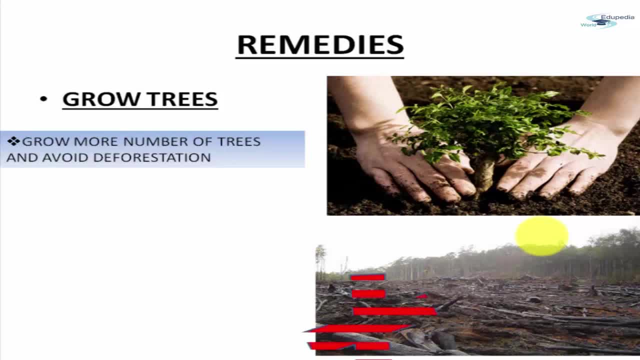 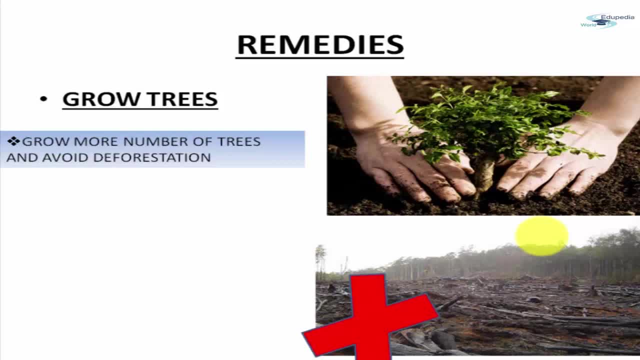